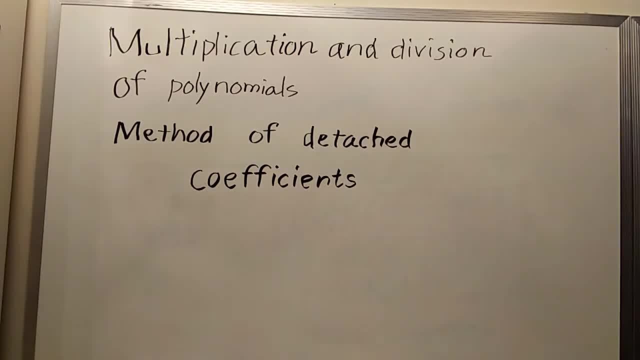 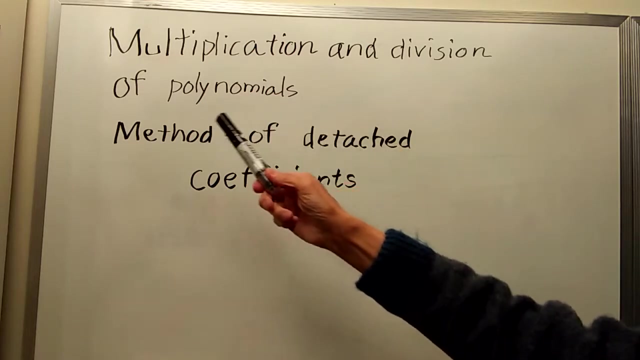 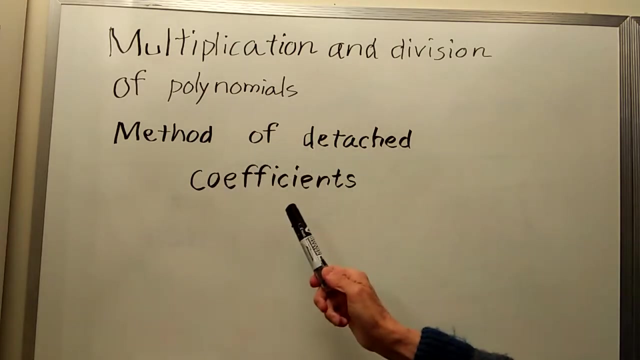 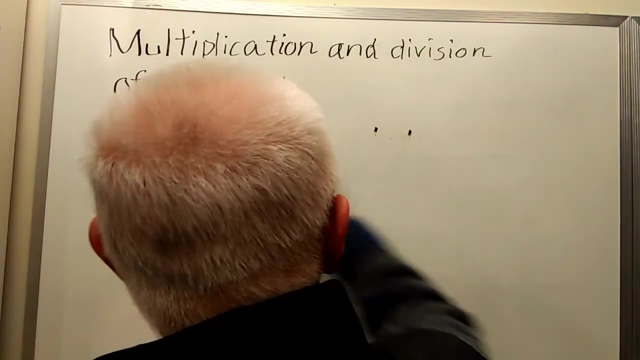 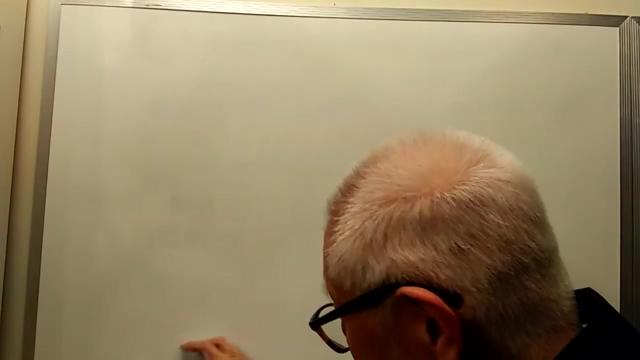 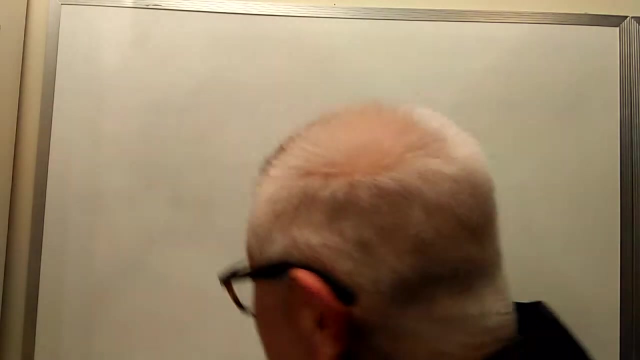 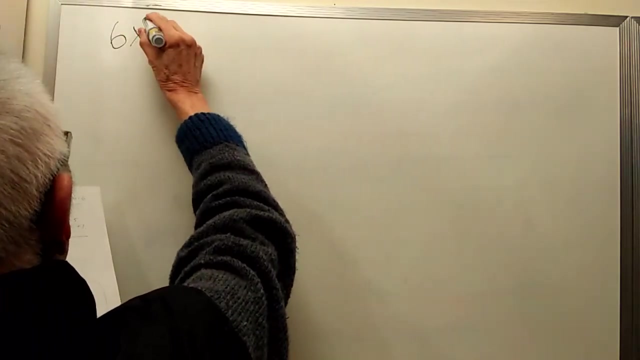 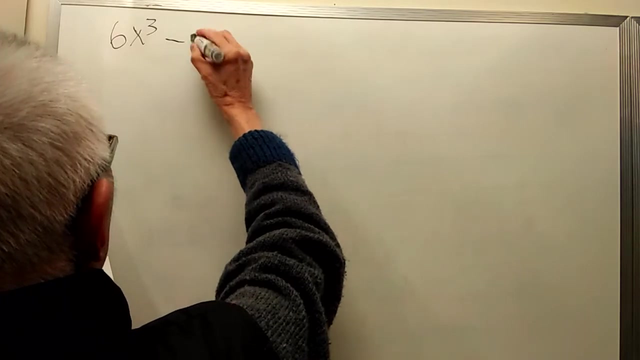 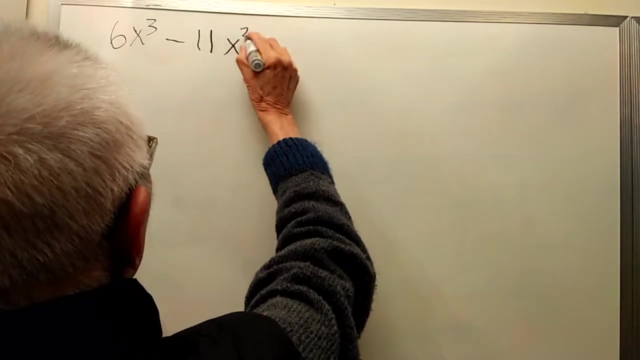 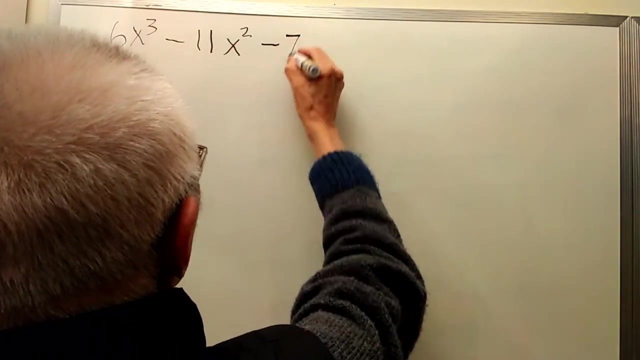 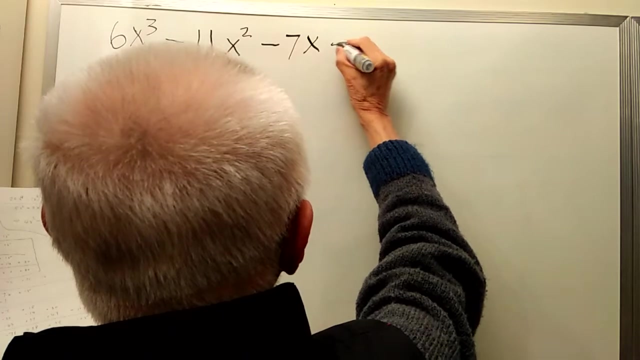 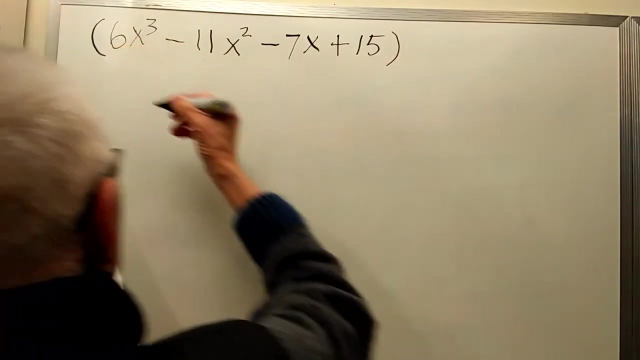 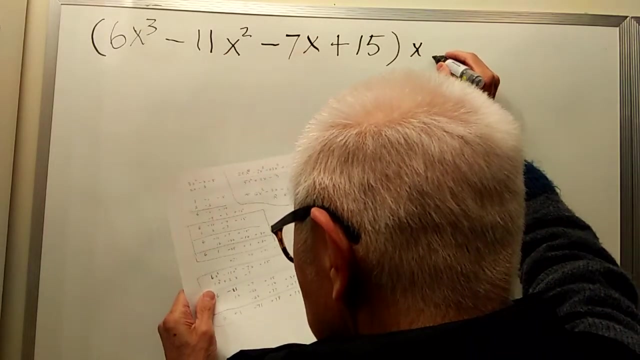 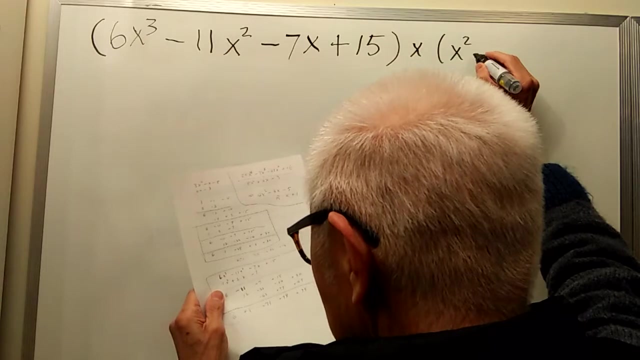 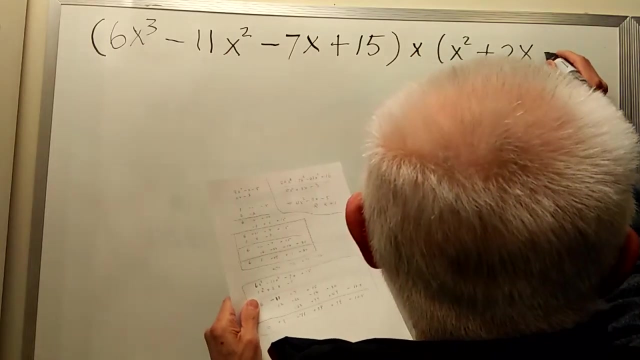 Multiplication and division of polynomials. Method of detached coefficients: 6x cubed Minus 11x squared Minus, 7x Plus 15.. This Times X squared Plus 2x Minus 7.. 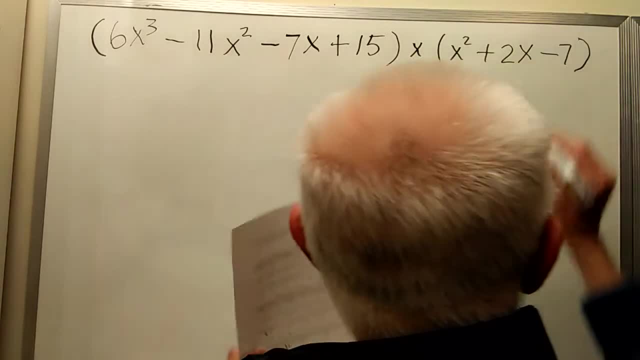 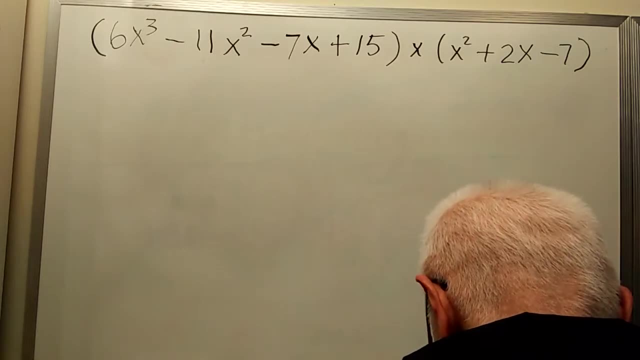 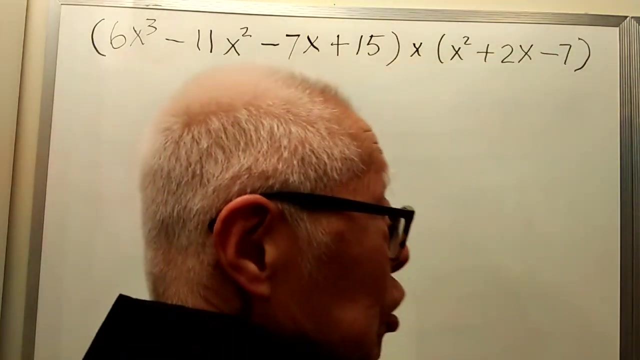 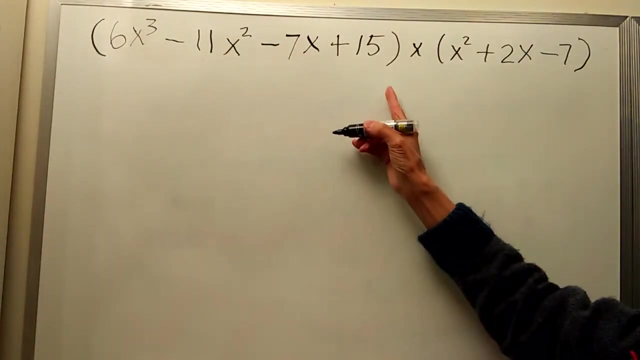 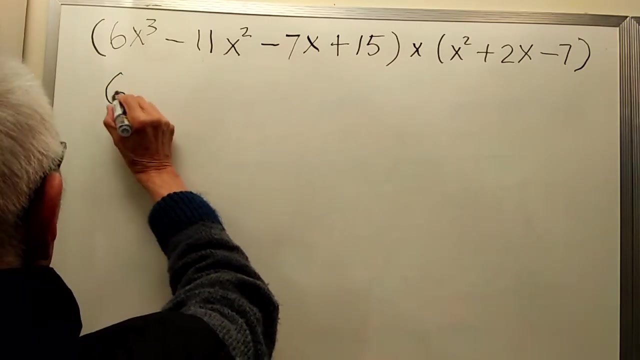 Okay, Let's use detached coefficients method. We write only the coefficients without writing x. Let's do it: 6x cubed Minus 11x squared Minus 12x squared Minus 12x squared Minus 12x squared. 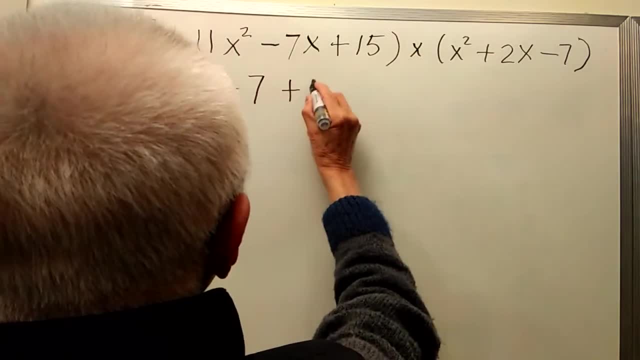 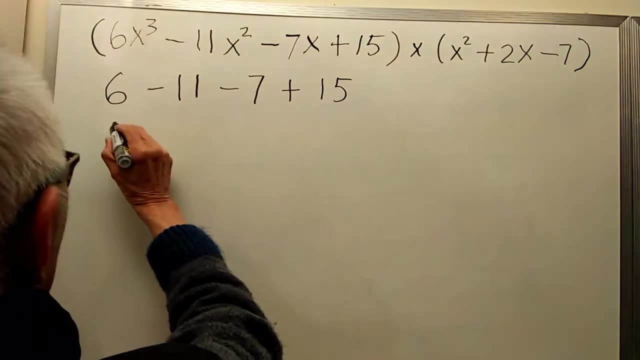 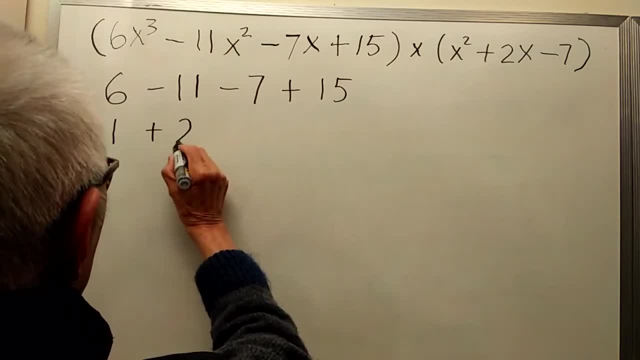 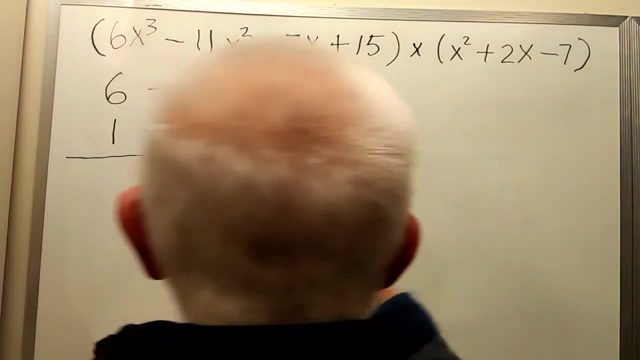 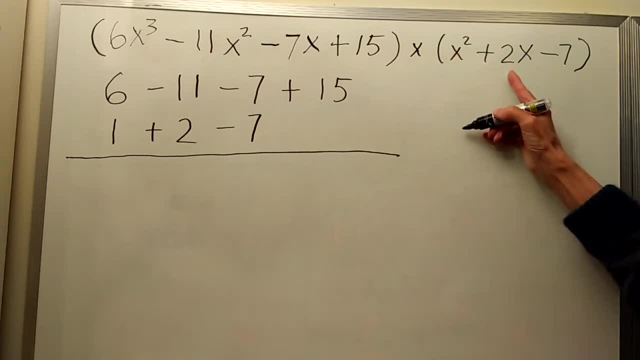 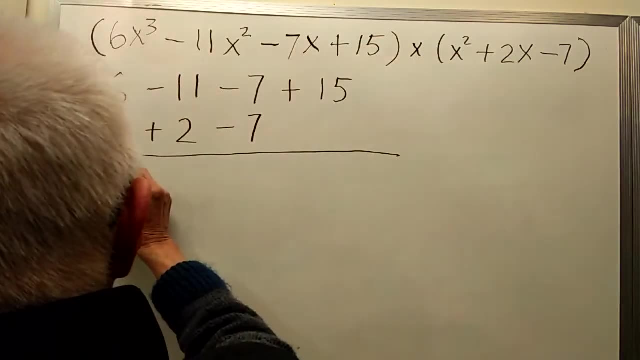 בשว asacą. y3eg2 accounts terms inning. given this 아��� temples polynomial, I only write 1,, 2, and minus 7.. Let us multiply: 1 times 6 is 6.. 1 times 11.. 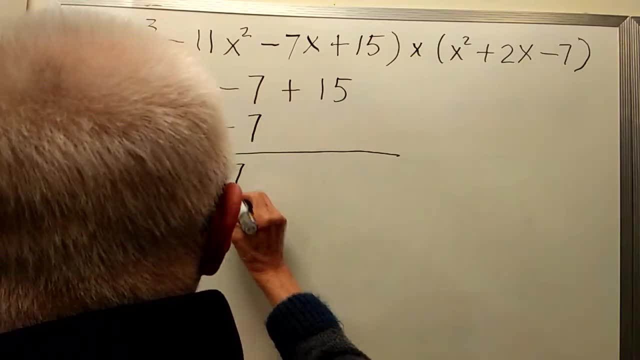 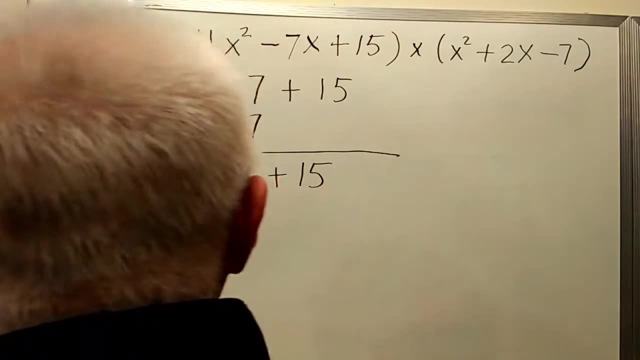 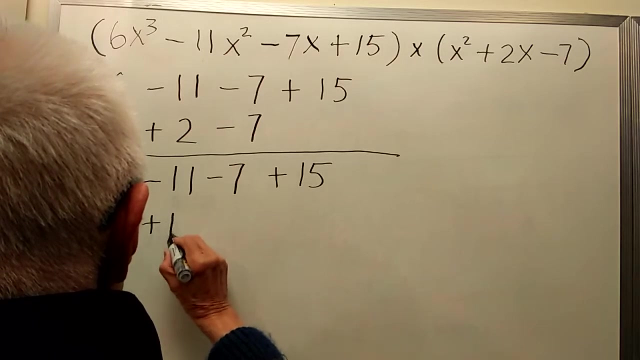 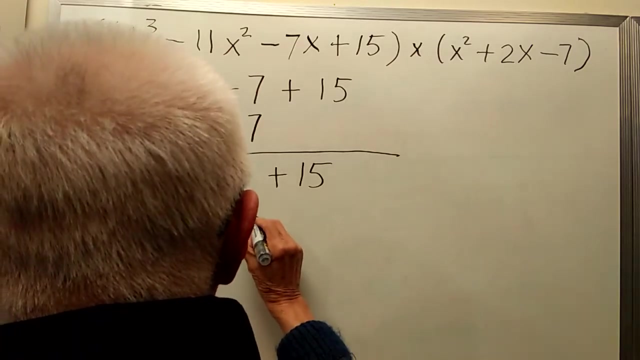 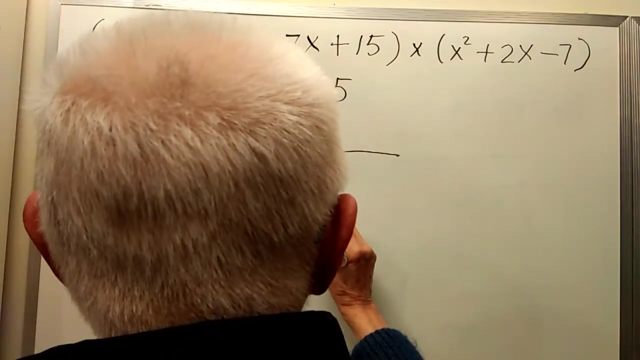 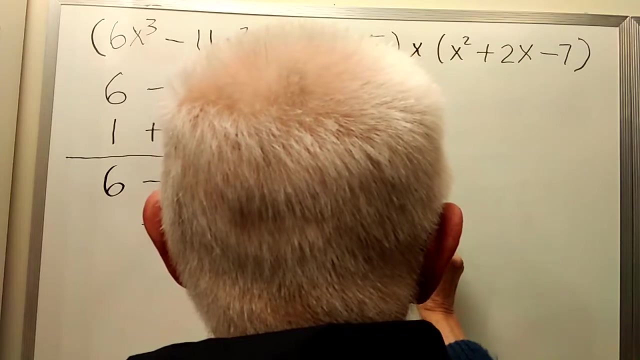 1 times negative, 7.. 1 times plus 15.. Okay, 2 times 6.. 2 times negative: 11.. 2 times negative: 7. 2 times 15.. 2 times negative: 7.. 7 times 6.. 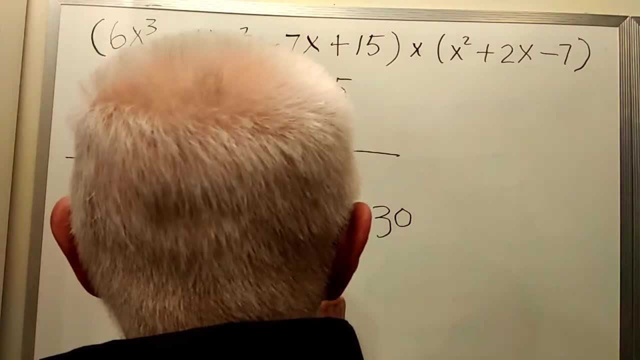 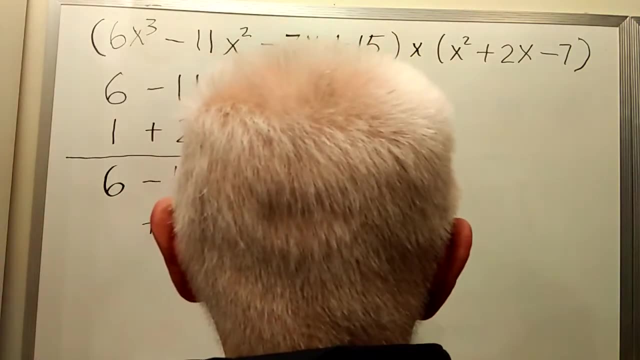 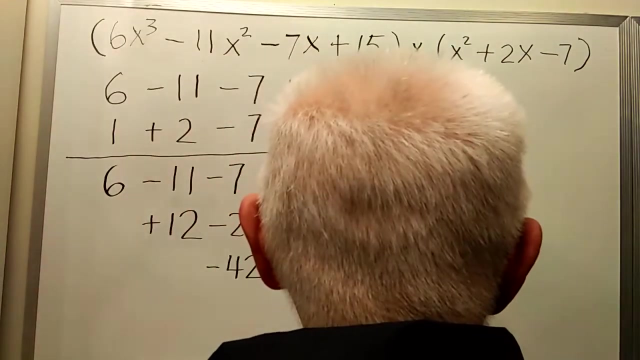 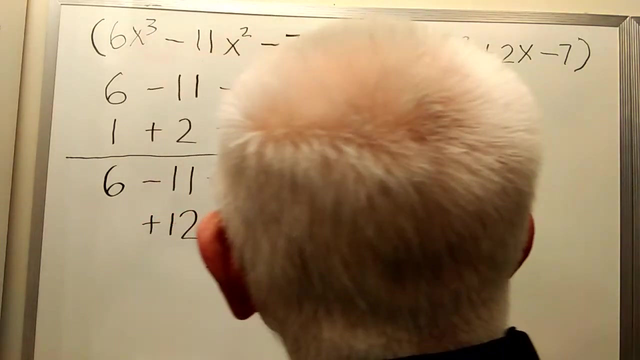 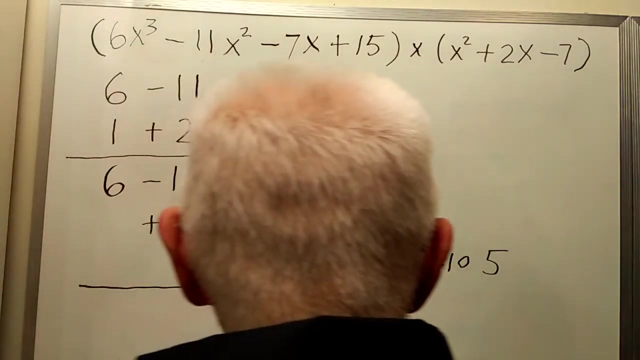 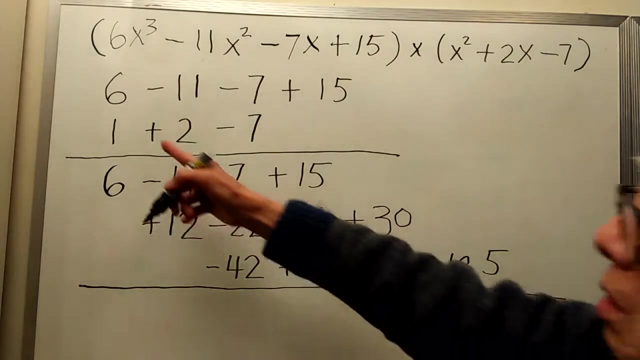 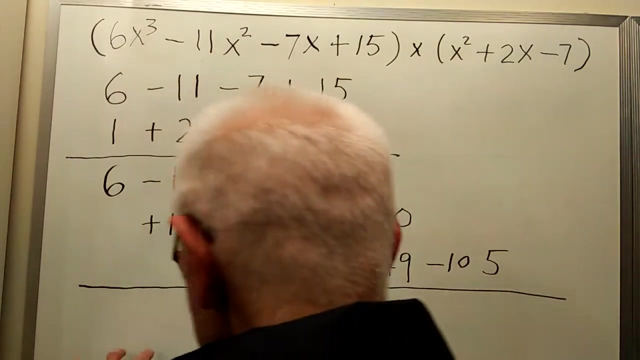 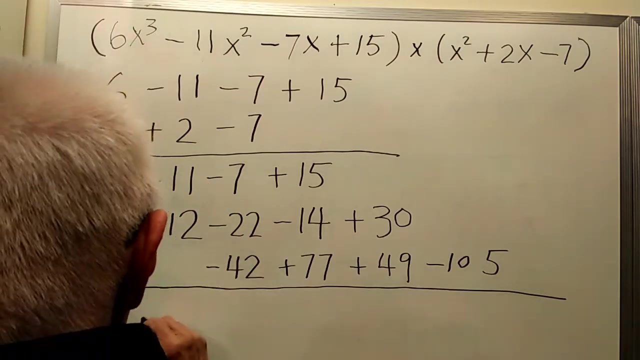 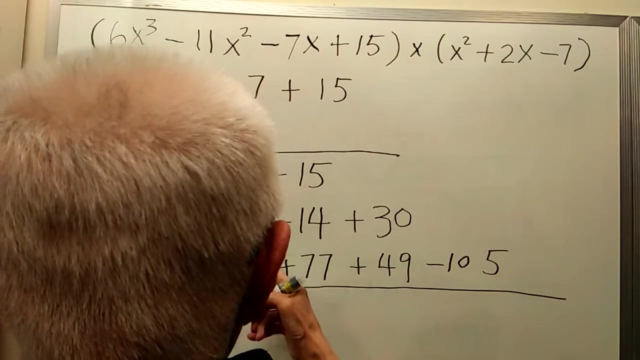 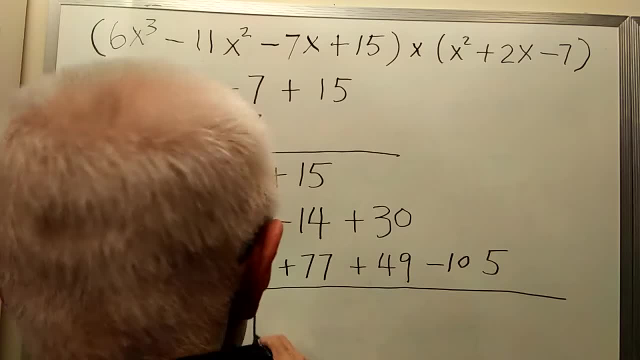 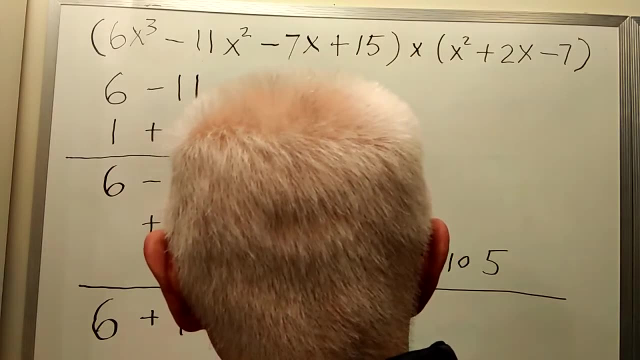 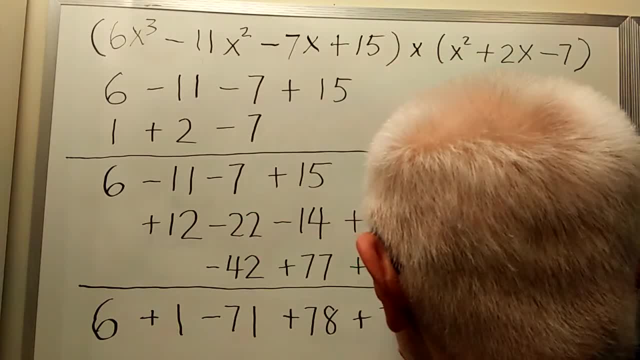 1,, 2,, 3,, 4,, 5,, 6,, 7,, 8,, 9, 10.. Add here: 1,, 2,, 3,, 4,, 5,, 6,, 7,, 8,, 9,, 10, 10.. 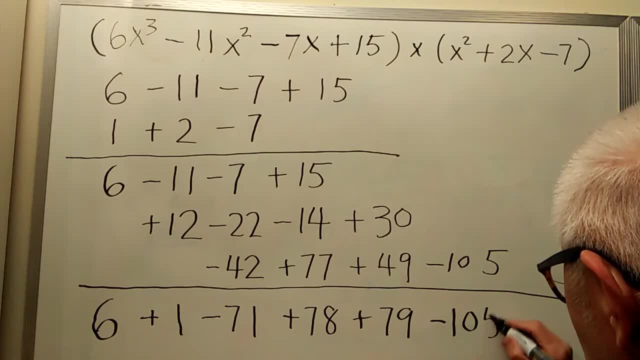 Add here 1,, 2,, 3,, 4,, 5,, 6,, 7,, 8,, 9, 10.. Add here 1,, 2,, 3,, 4,, 5,, 6,, 7,, 8,, 9, 10.. 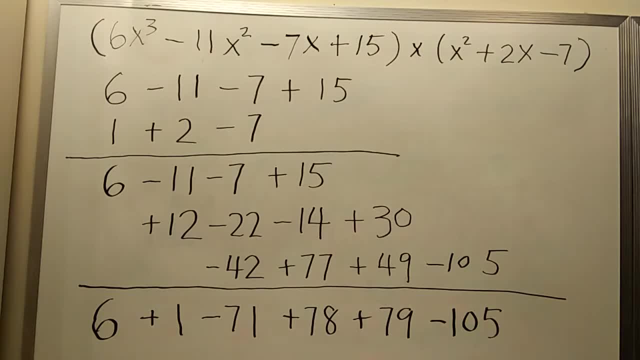 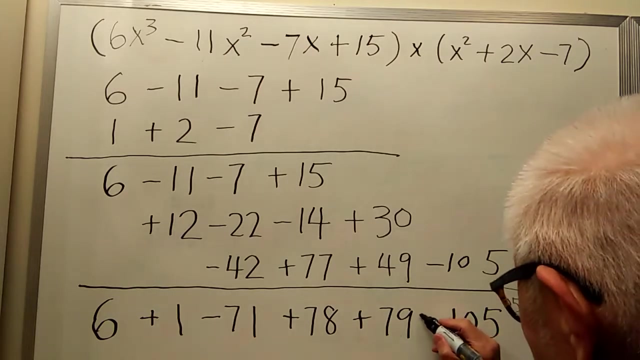 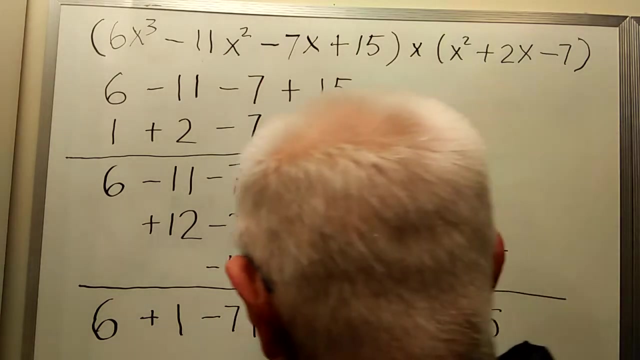 Add here. So we used the method of detached coefficients. Our final result contains only the coefficients. So the final step is to add x to this line. This is x to the power zero. this is x to the power one and power two, power three, power four, power five. So let's add x. 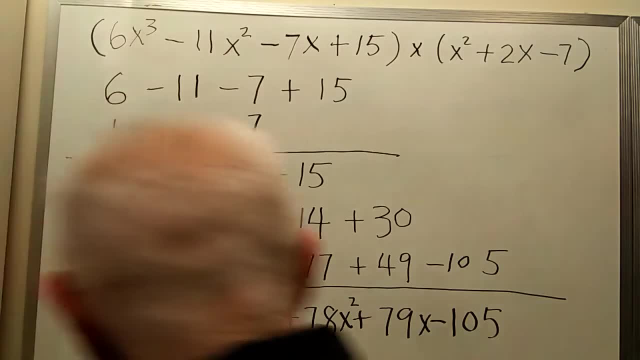 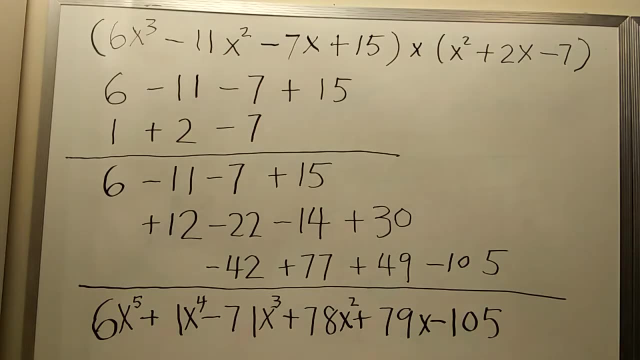 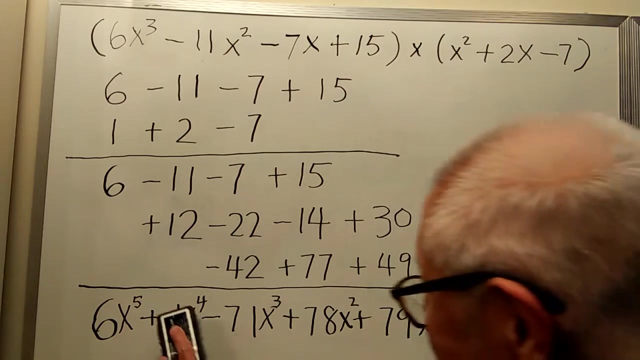 Now, this is our final answer. So it's x, x squared, x cubed, x to the power four, x to the power five. I do not need to write one x to the power four, so I just erase a one. This is my final answer. 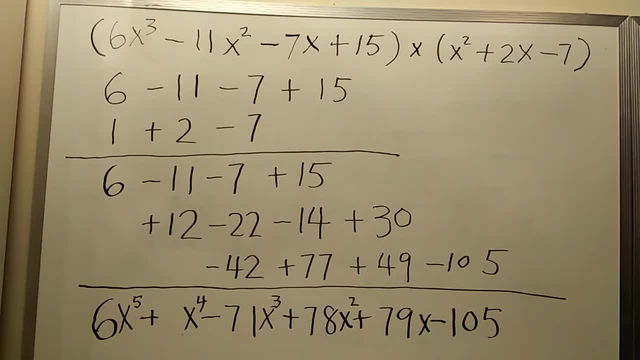 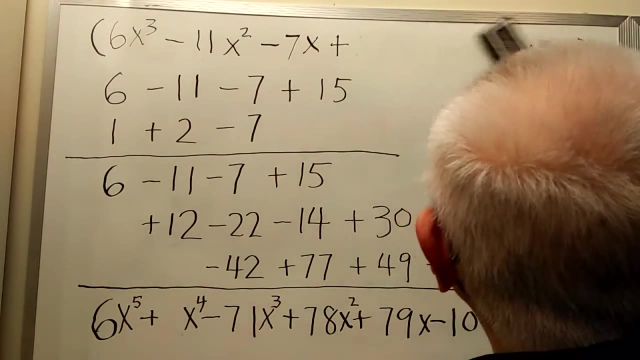 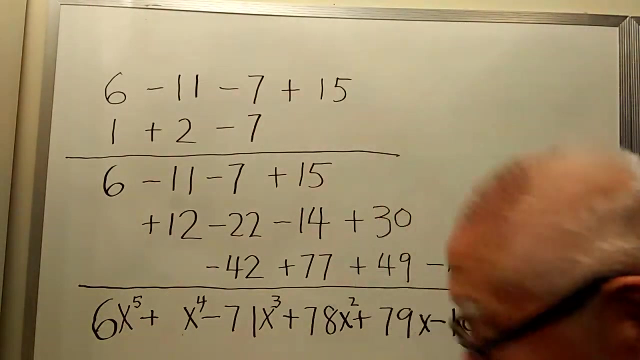 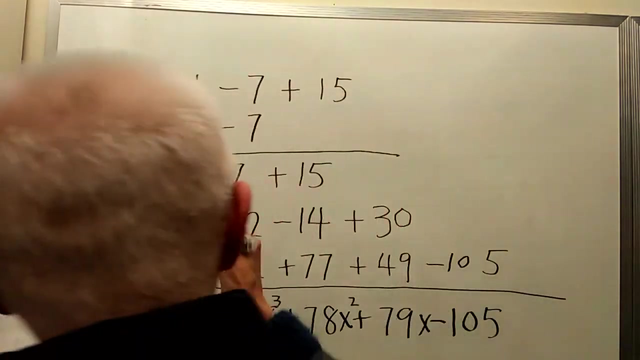 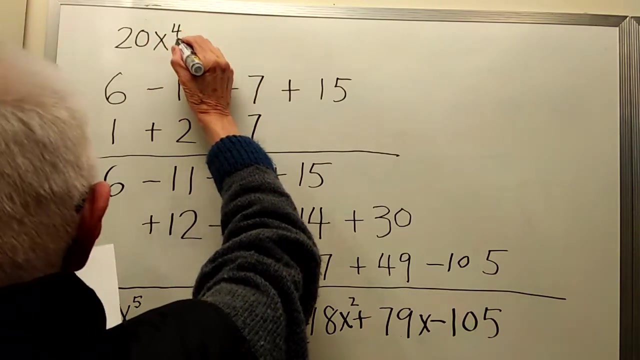 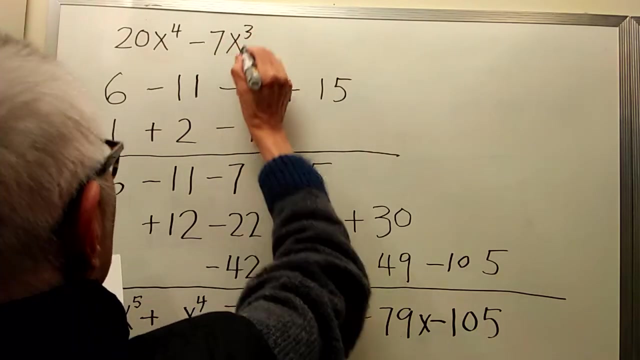 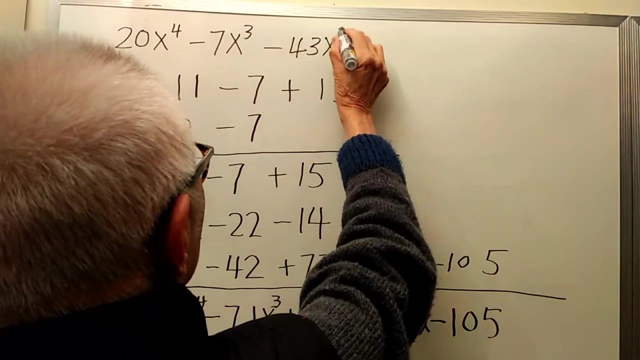 Next example is to do the division. We can use the same method of detached coefficients. You take your 17th sermon and divide it by the end result. Question mark 1.. Question mark two. Question mark three. Question mark four. Question mark five. 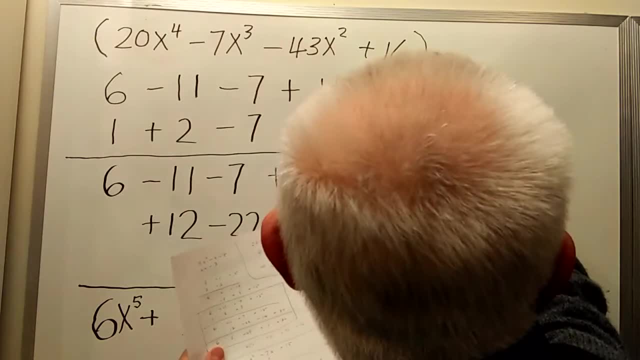 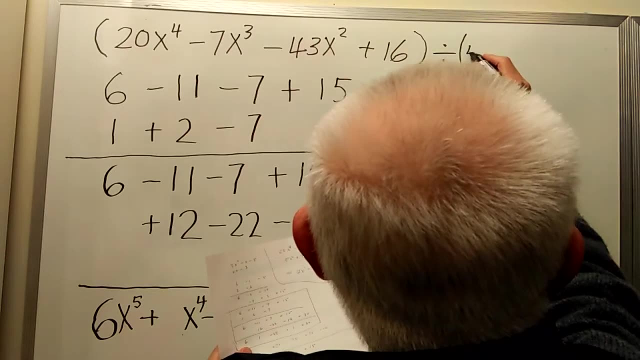 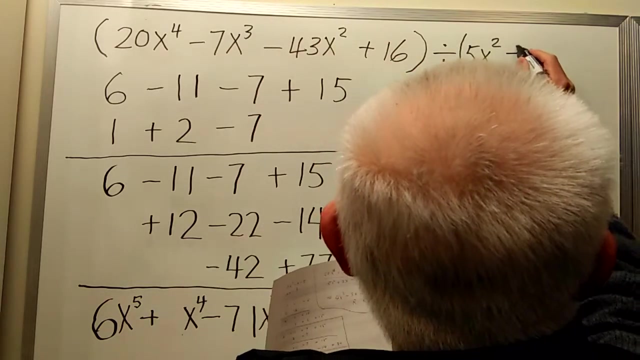 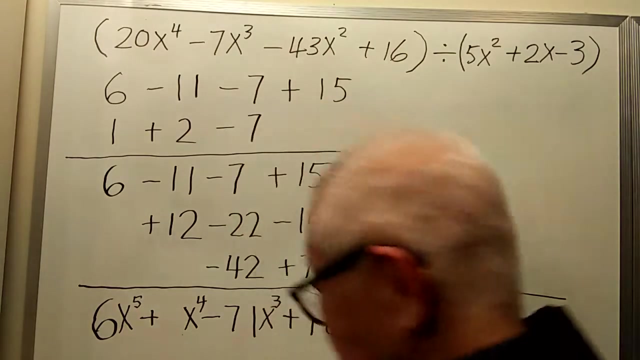 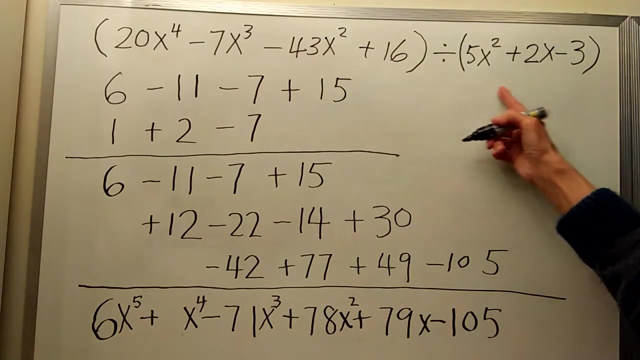 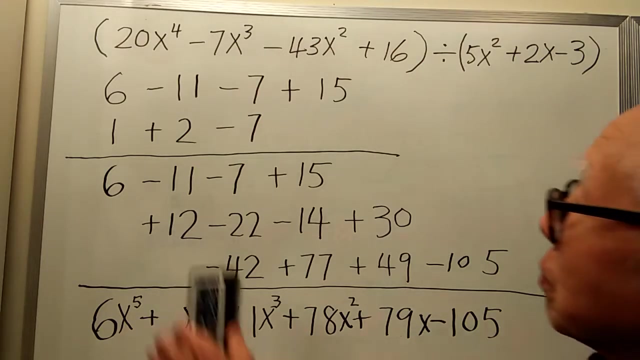 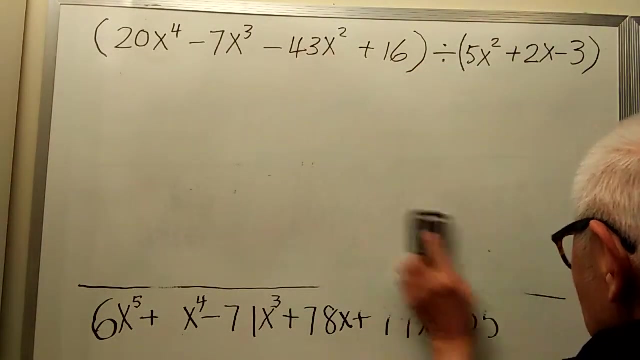 Question mark six. Question mark seven. Question mark nine. Question mark 10.. We have one polynomial divided by another polynomial. Let's use the same method: detached coefficients. We write only the coefficients, without writing x. Okay, Okay, Okay. 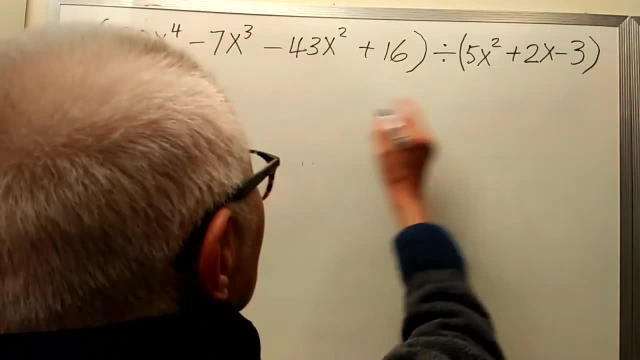 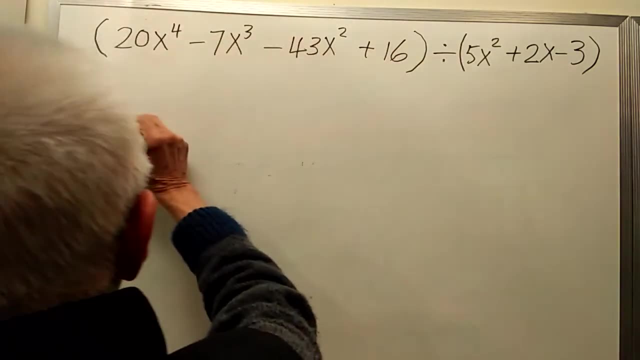 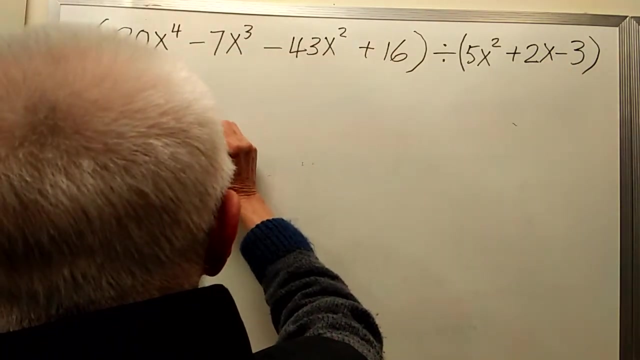 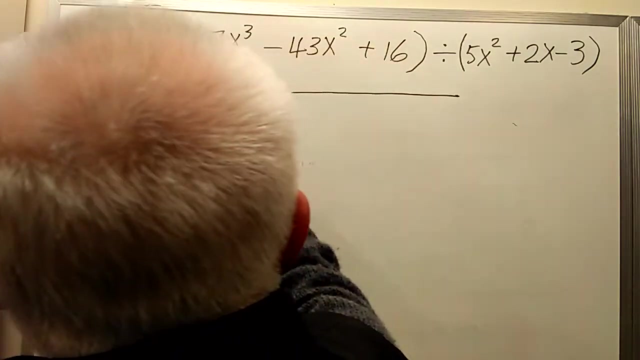 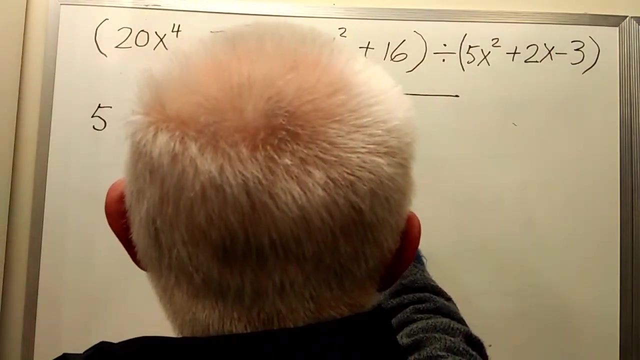 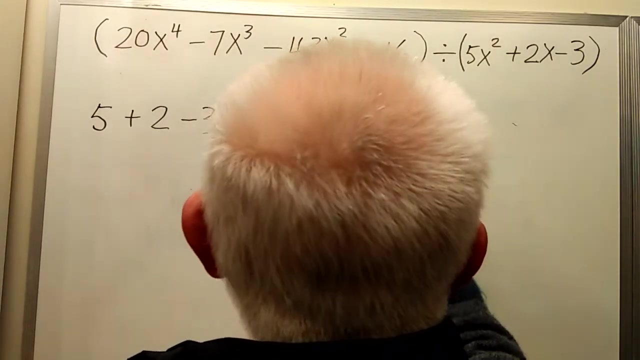 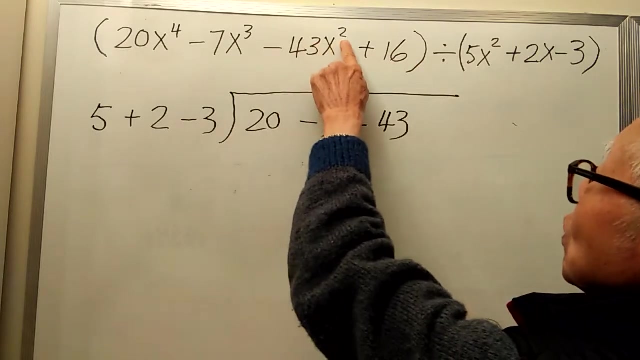 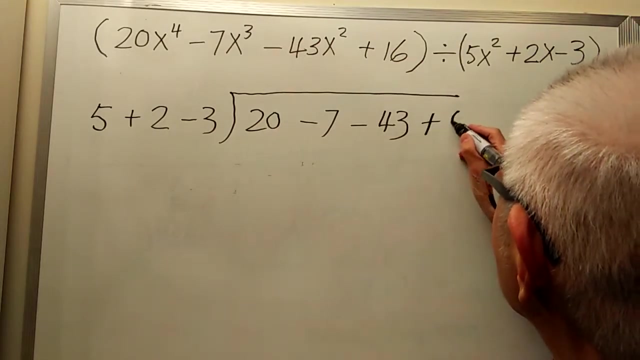 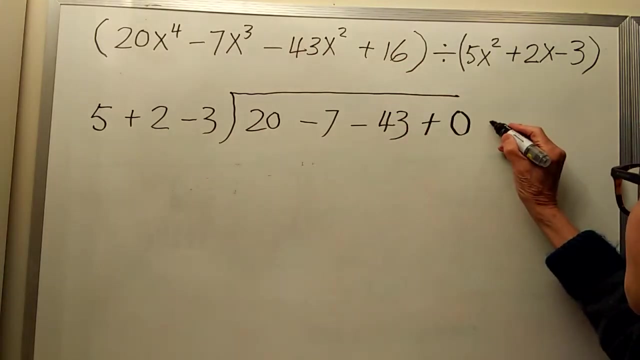 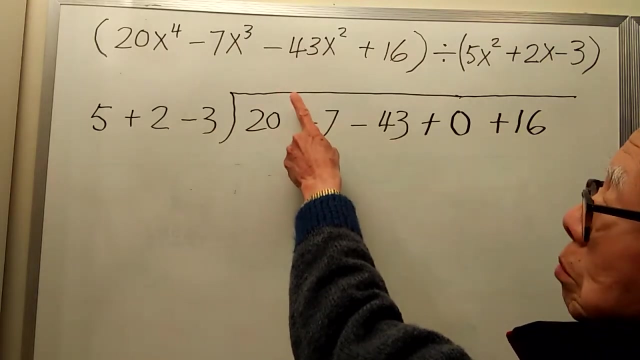 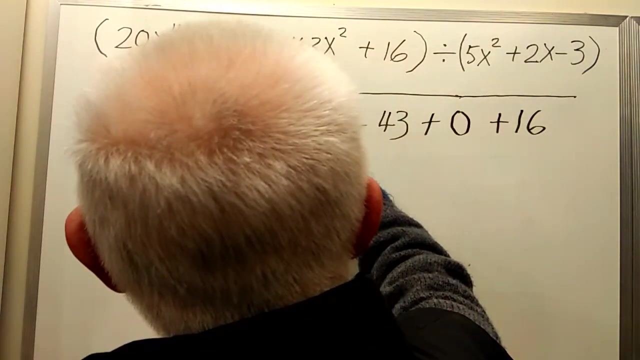 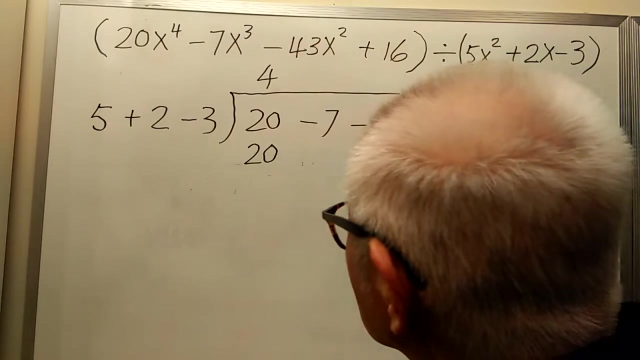 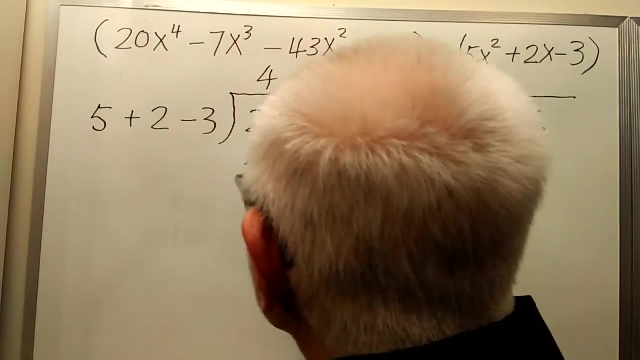 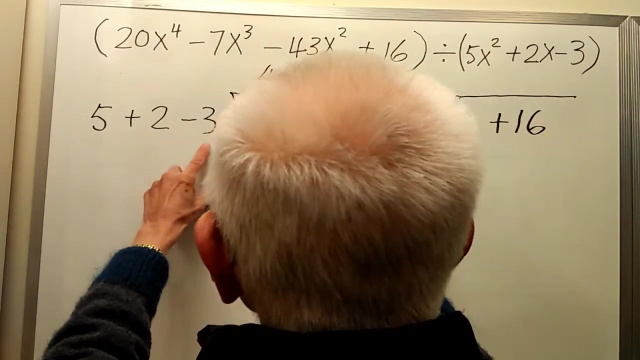 Okay, Okay, Whoops. Four, three, two. I am missing the x term. The zero represents I have no x term. Okay, now we do it. What times 5 gives you 24?? Two times 4 is 8.. 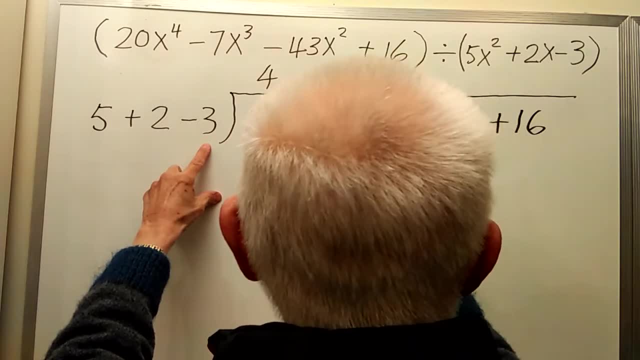 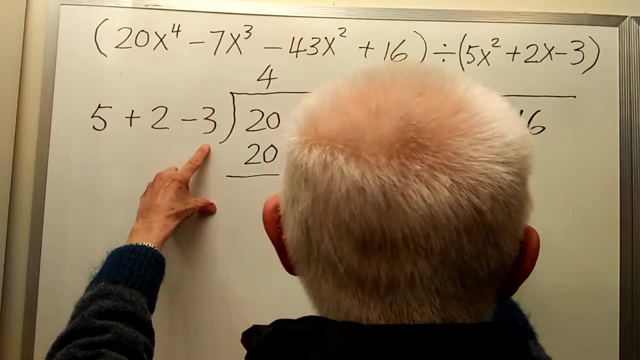 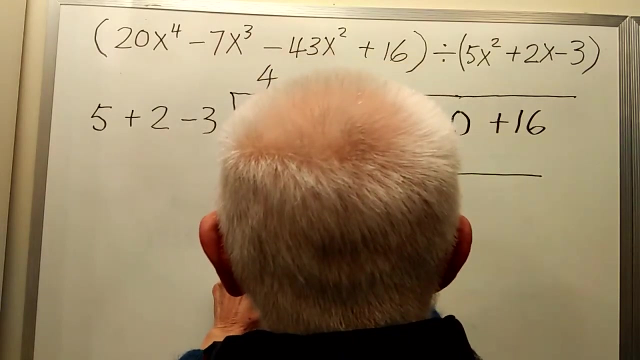 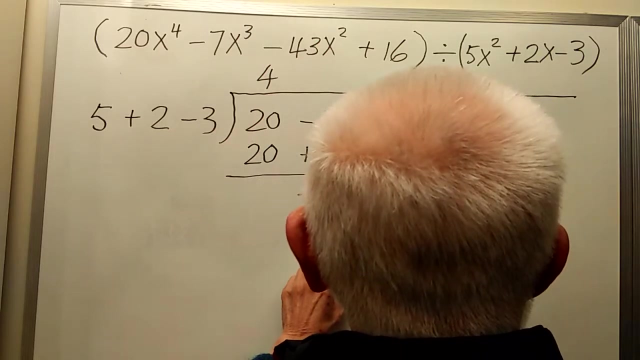 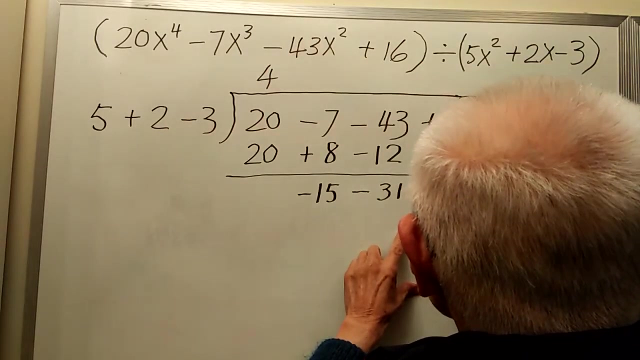 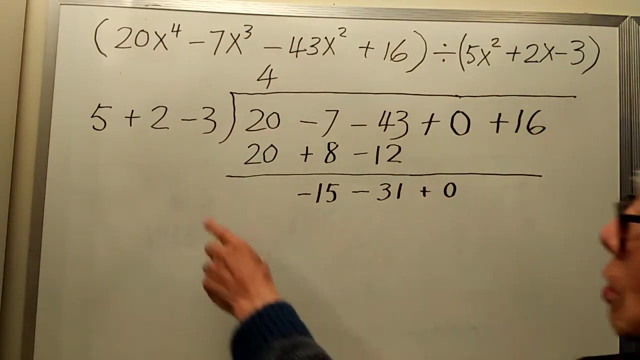 Three times 4 is 8.. Two times 4 is 8.. Three times 4 is negative 12.. We subtract This is 0.. Subtract, Subtract, Subtract, Subtract, Subtract. Alright, What times 5 gives you negative 15?? 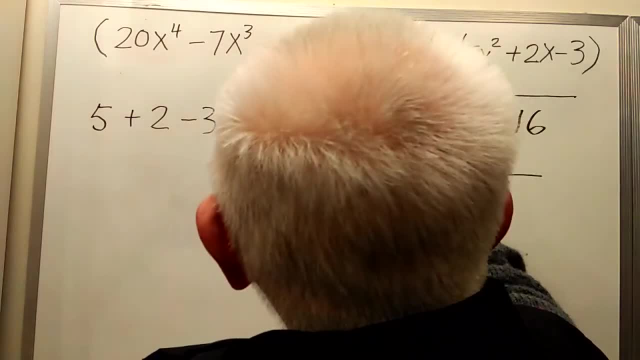 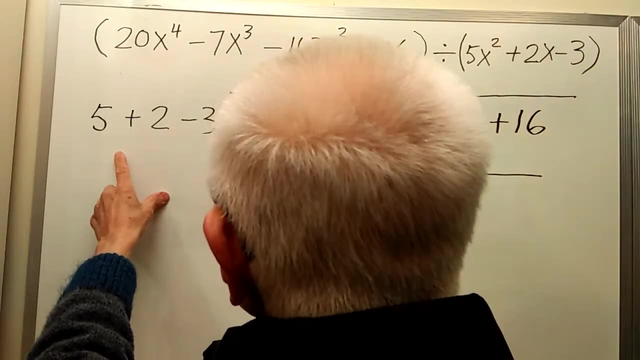 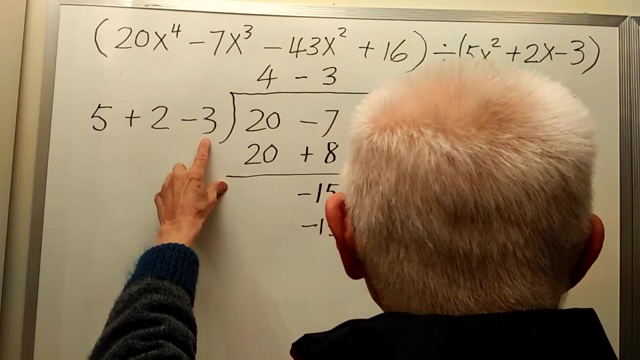 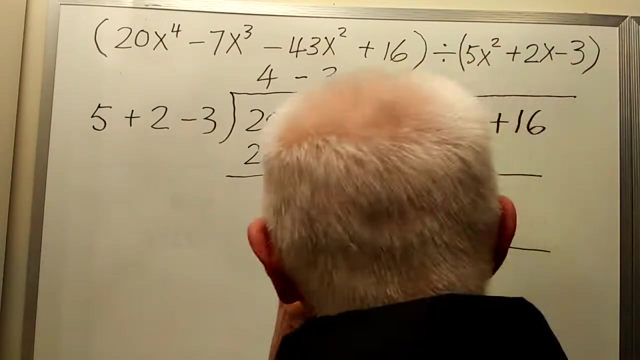 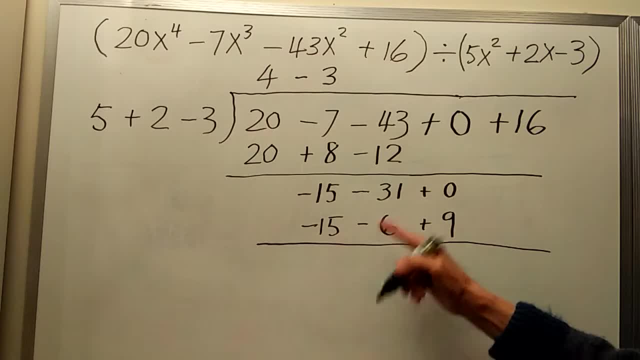 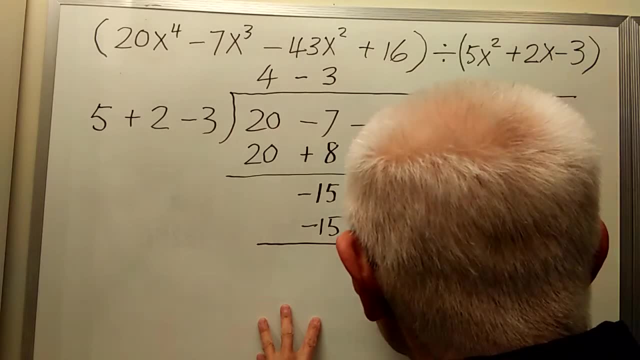 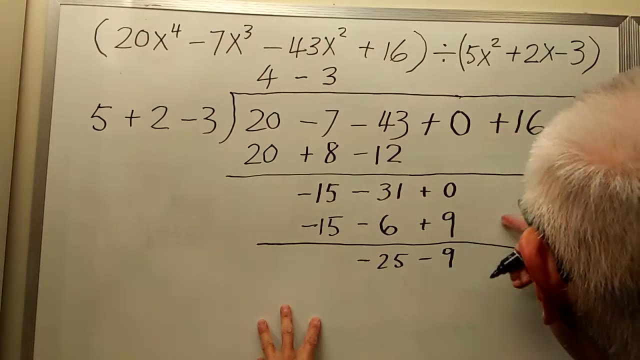 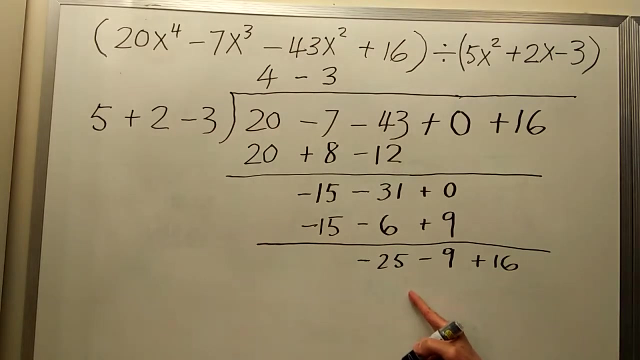 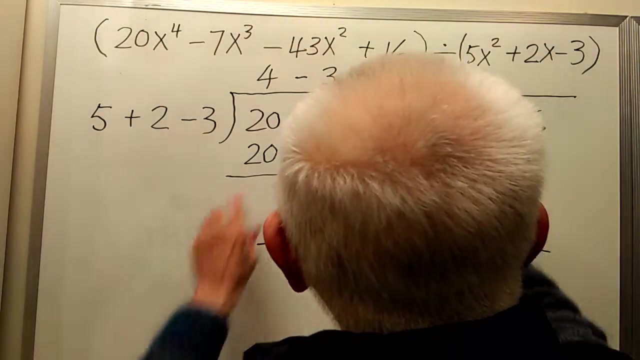 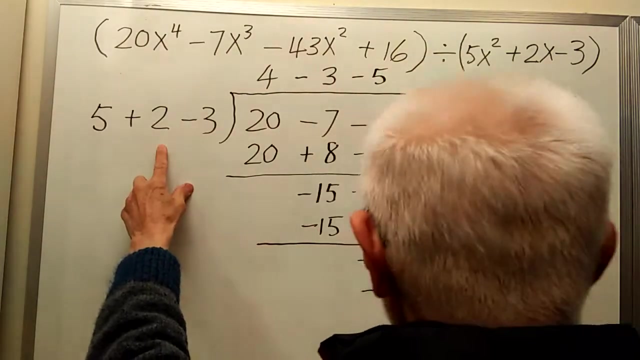 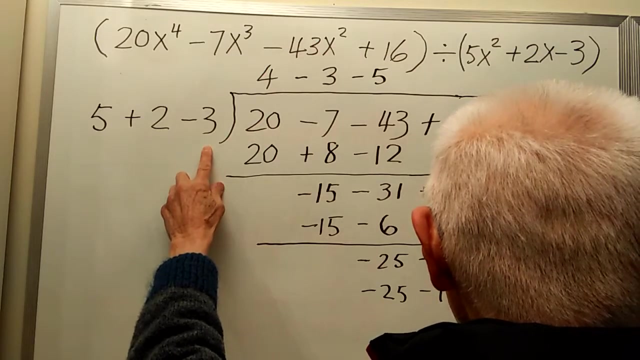 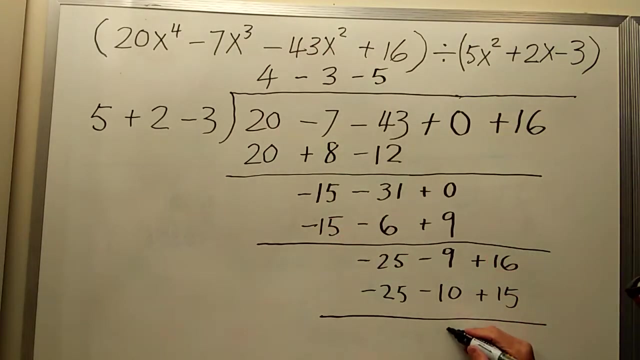 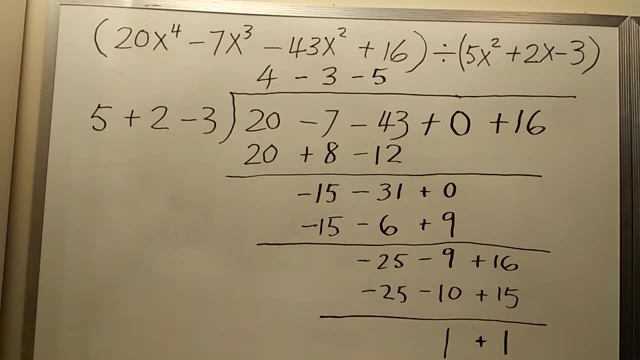 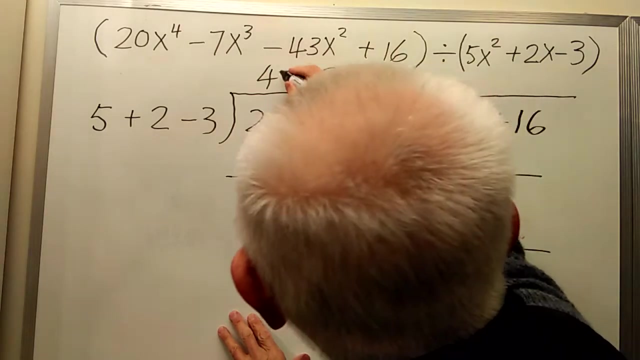 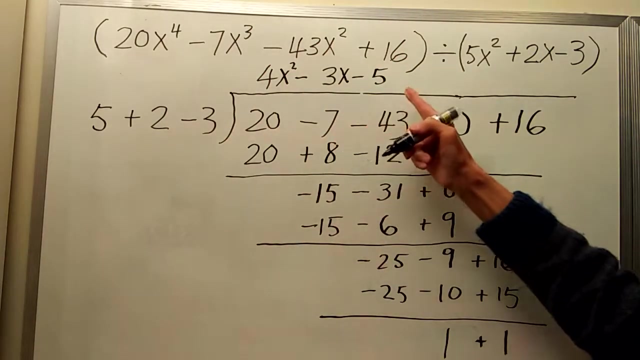 Now, like what we did for the last example, the multiplication, now we need to add x to our result, because our result contains only the coefficients. This is 0x. this is x to the power 1, and this is x squared. this is x. this has no x. 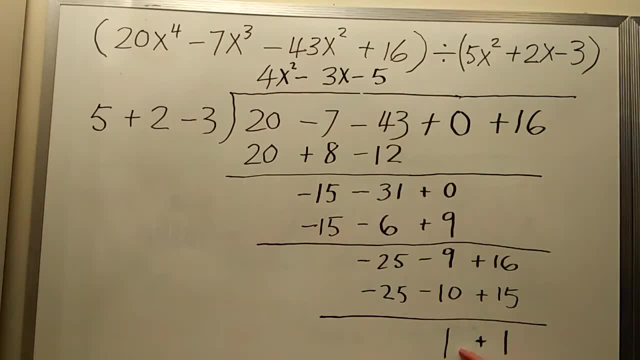 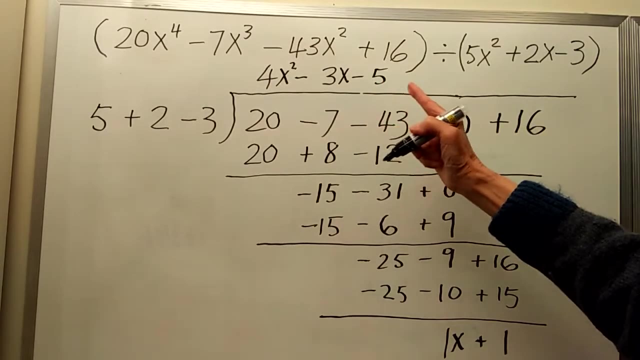 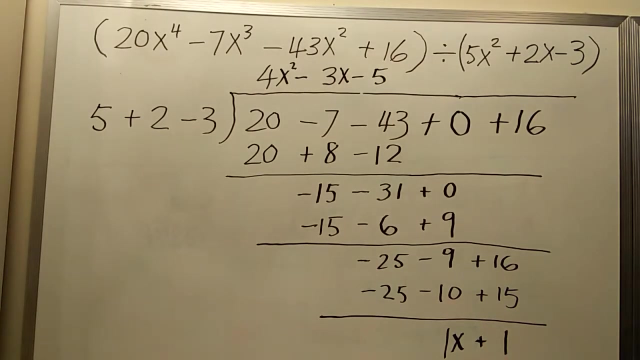 This has no x, this is x. So our result is: the quotient is 4x squared minus 3x minus 5, and the remainder is 1x plus 1.. I don't need to write the 1,, so I can erase the 1.. 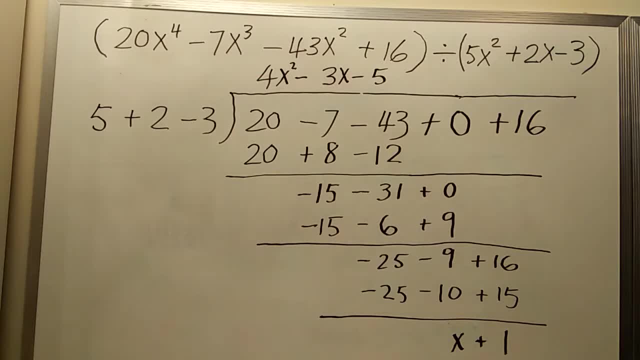 The remainder is just x plus 1.. This completes today's video. Multiplication of polynomials and division of polynomials using the method of detached coefficients. Thank you for watching. Goodbye, We will do the next video soon. Thank you. 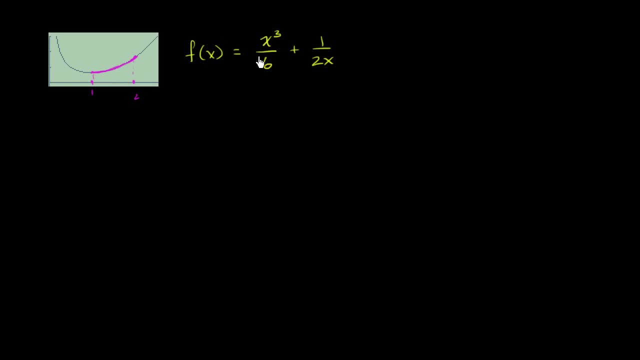 This right here is the graph of y is equal to x, to the third over six, plus one over two x. What I want to do in this video is figure out the arc length along this curve between x equals one and x equals two, And so we've already highlighted that in this purplish color. 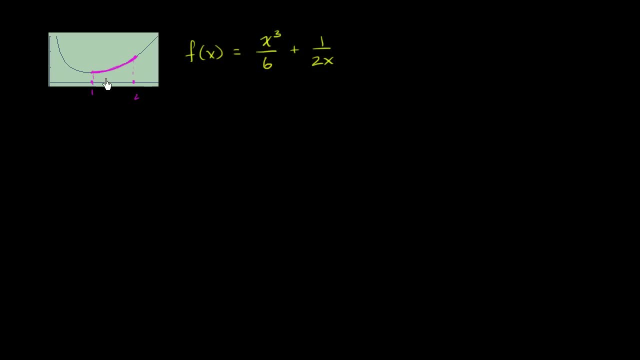 So I encourage you to pause this video and try it out on your own. And I'll give you one hint: Assuming that you apply the arc length formula correctly, it'll just be a little bit of power algebra that you'll have to do to actually find the arc length.